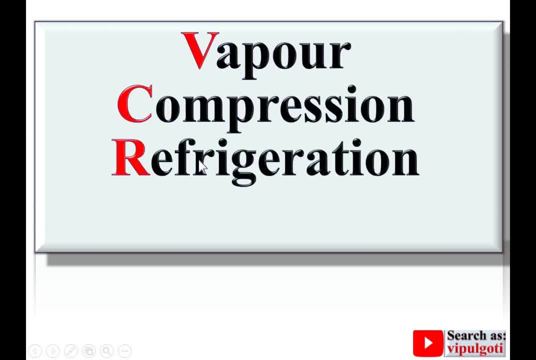 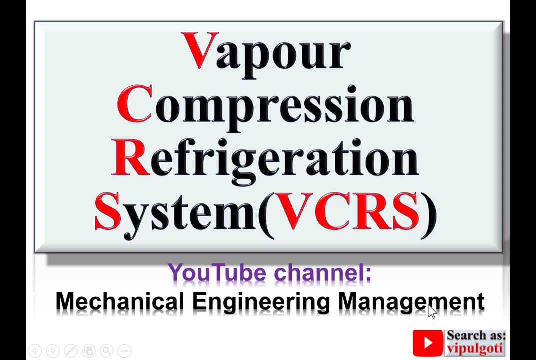 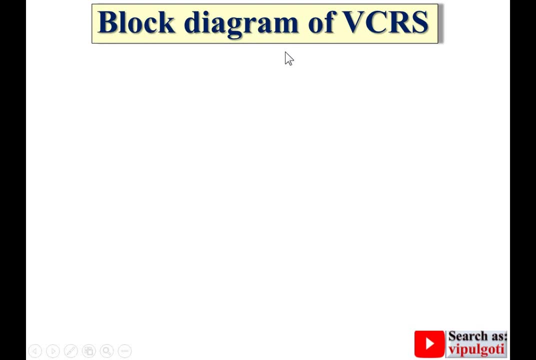 Today we are going to discuss about vapor compression refrigeration system and the short form, VCRS. So welcome to my youtube channel, mechanical engineering management. So first of all, try to understand the block diagram of VCRS, because of sometimes in the examination it can be separately asked to draw only the figure of the VCRS. 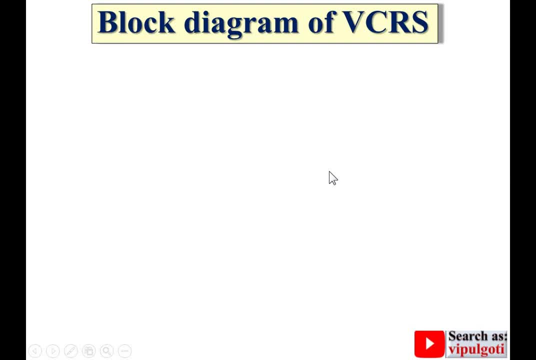 But before starting the block diagram of VCRS, first see the different component of the VCRS. So first compressor, then second one is the condenser, third one is the expansion valve and fourth one is the evaporator. So first assume this is the straight one and this component is the compressor. 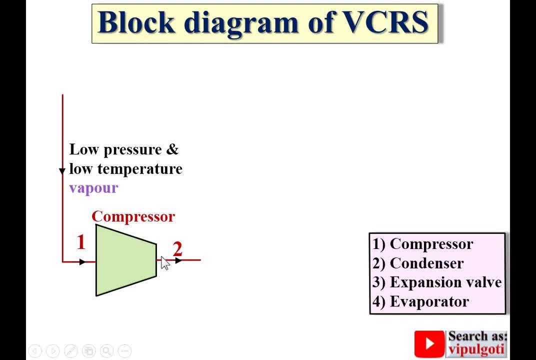 and this is 2, that means during the 1-2 process, low pressure and low temperature vapor is converted to VCRS. So in this process the vapor is converted into high pressure, high temperature vapor and this vapor is what actually refrigerant vapor. So during the 1-2 process, the pressure, 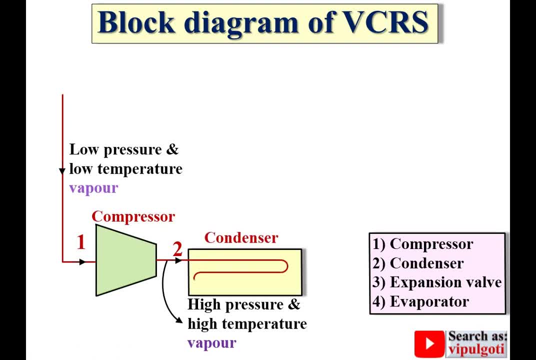 and temperature. both will increase Now. next it will pass through the condenser, So let's say it is the 0.3. So during the process 2-3 it passes through the condenser where it rejects the heat to the atmosphere, and at 0.3. 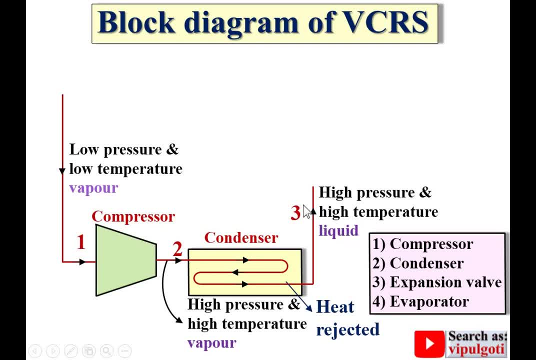 high pressure, high temperature liquid. During the process 2-3, high pressure, high temperature vapor is converted into high pressure, high temperature liquid. So keep in mind that vapor is converted into the liquid. Then it will pass through the expansion valve And let's say it is the point number 4.. During 3-4, the refrigerant will expand to the expansion. 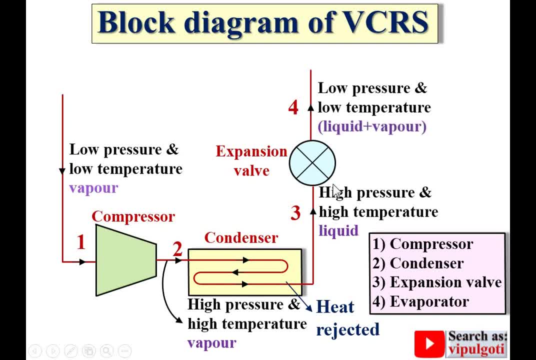 valve and so that the high pressure, high temperature liquid is converted into low pressure, low temperature mixture of liquid and vapor, And then it will pass through the evaporator. So evaporator also consists the tubes where the heat is exchanged from the refrigerant to the space of the evaporator. So evaporator and condenser, both are actually. 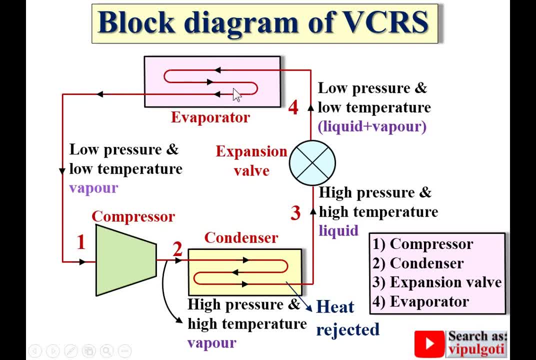 one type of the heat exchanger In the evaporator. refrigerant absorbs heat, So I can say heat absorbed in the evaporator by the refrigerant And so that the mixture of liquid and vapor is converted completely into vapor. So this is the block diagram of the VCRS. 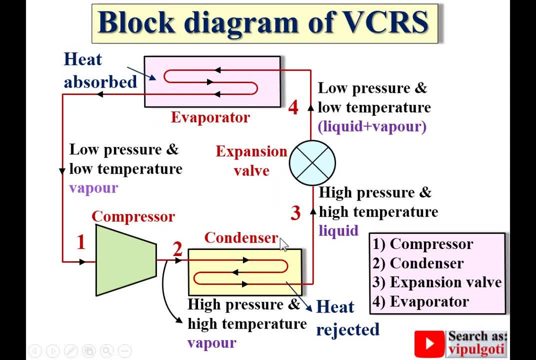 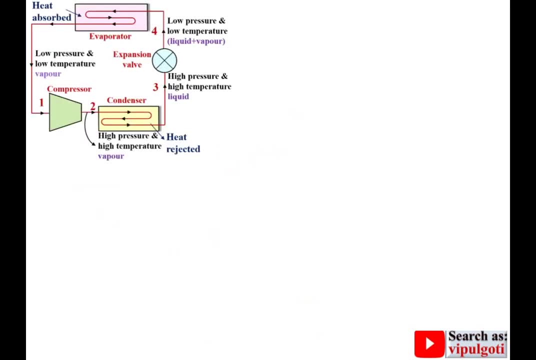 So I think you can understand now the flow of the refrigerant and the different component of the vapor compression refrigeration system. Now we will discuss the same VCRS with the help of this block diagram in detail. So this is. earlier we have seen block diagram of the VCRS And now we are. 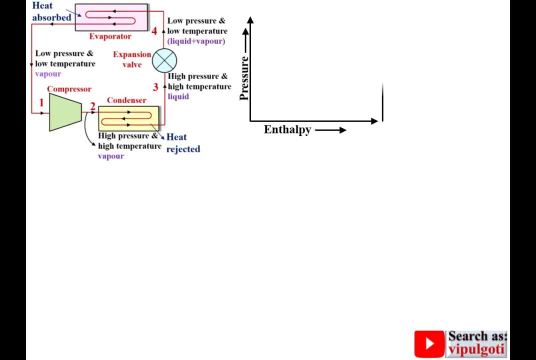 going to discuss that VCRS with the help of the pressure enthalpy diagram and temperature and entropy diagram. So sometimes it is called as the PH diagram and this is called as the TS diagram. And this is the saturation curve on the pressure versus enthalpy diagram. 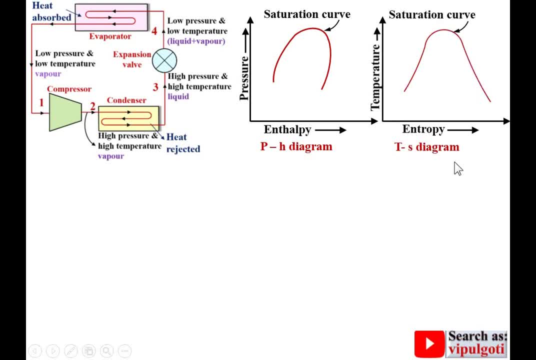 And this is also saturation curve on temperature entropy diagram. Saturation curve that means the left side of that saturation curve that means in this zone it is a liquid, and right side of this saturation curve that means in this zone it will be vapor, Whereas in this dome that means in the saturation curve it is a mixture of vapor and liquid. 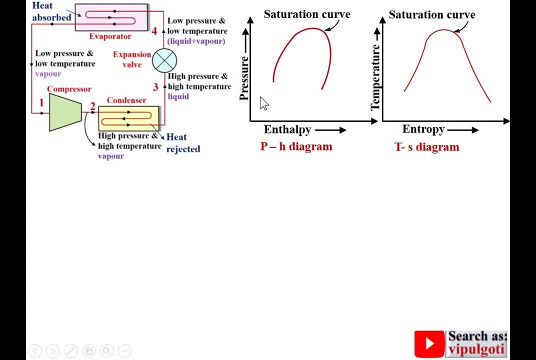 Similarly over here. So in the examination, if I want to draw the pressure enthalpy diagram as well as temperature entropy diagram, First you have to draw the saturation curve Because of with reference to that you can understand the VCRS. So first I am going to consider the 1-2 process. So during 1-2 process, what happen? 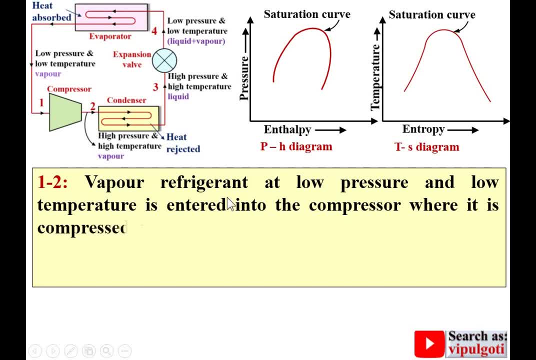 So the refrigerant will pass through the compressor, So vapor refrigerant at low pressure and low temperature is entered into the compressor, where it is compressed to high pressure. So here you can see, So that the temperature of vapor refrigerant is also increased. So that is high temperature. 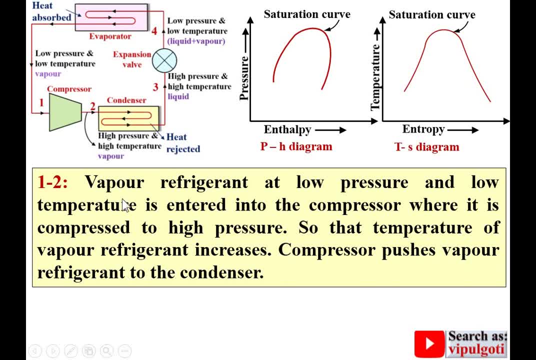 compressor pushes vapor refrigerant to the condenser, Then high temperature, high pressure vapor refrigerant is entered into the condenser. and if I want to show the same 1-2 process on this pH diagram, then it will be like that 1-2 process and you know that it is actually. 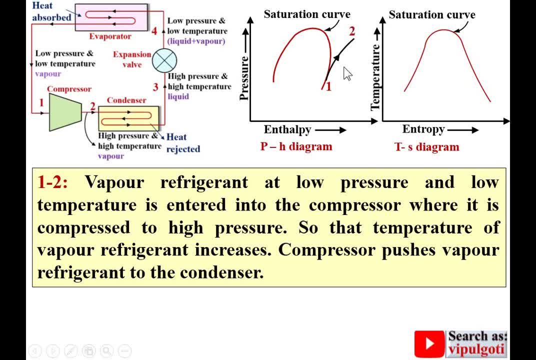 compressed. that's why it is called as adiabatic compression and on the TS diagram it will be the straight vertical line, because of adiabatic process is considered as the isentropic process. that means entropy is constant and this is the entropy, so it should be the vertical line. 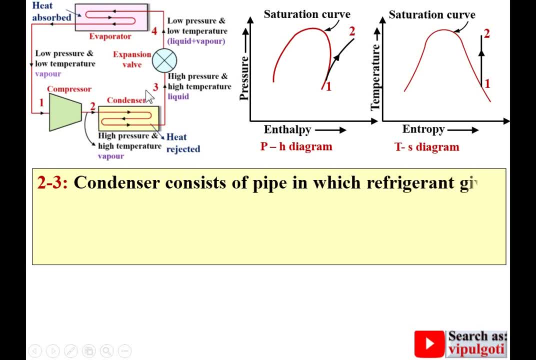 Next it will enter now in condenser, so I am going to consider 2-3 process. Condenser considers the adiabatic process, So I am going to consider 2-3 process. So I am going to consider 2-3 process. 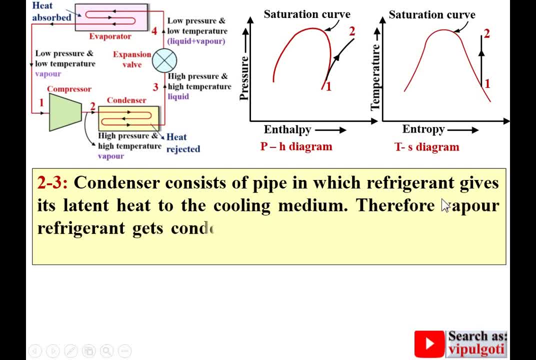 So I am going to consider 2-3 process. You can see over here. this is the pipe in which refrigerant gives it's latent heat to the cooling medium, and cooling medium is what actually The environment that means surrounding, therefore vapor refrigerant gets condensed in the condenser. 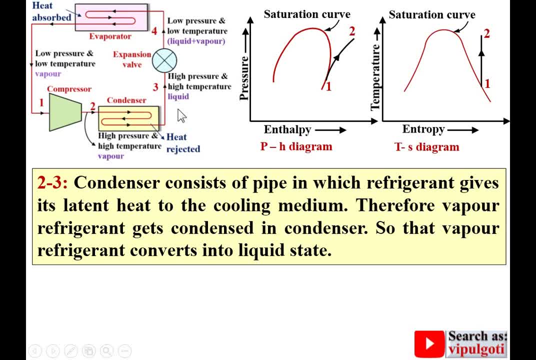 and here you can see that is condensed So that the phase is chained from vapor to liquid, so that vapor refrigerant converts into the liquid state. and if I want to show that 2, 3 process on pH diagram then it will be. 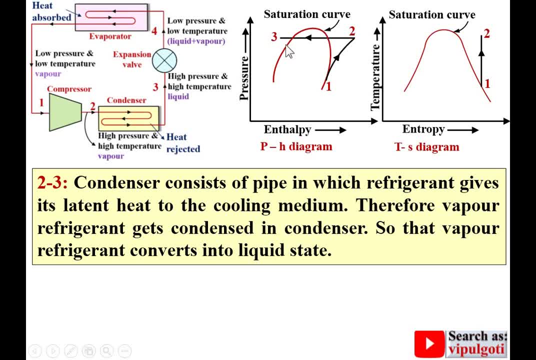 like that: at constant pressure, phase change from the vapor to the liquid phase. and on the TS diagram it is like that 2, 3 process. so first superheated refrigerant is up to the saturation curve and then phase change and up to the point 3 it will completely convert it into the liquid state. now next it. 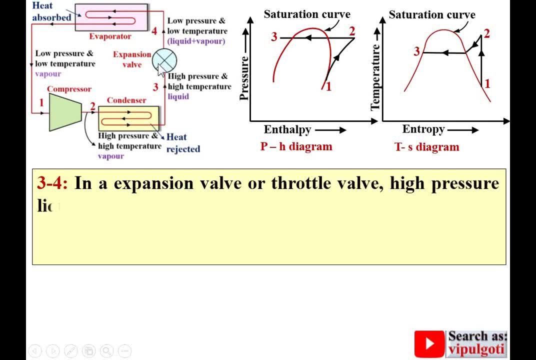 will enter into the expansion wall and that is the 3- 4 process. so in the expansion wall, or sometimes it is called as the throttle valve, high pressure liquid refrigerant is expanded to low pressure and low temperature. here you can see high pressure, high temperature liquid is expand and so that it will low. 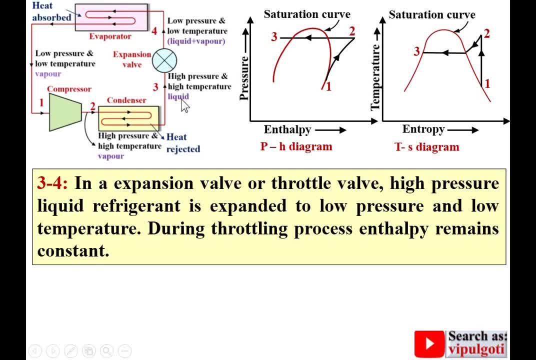 pressure, low temperature. but the important point is what. the liquid is converted into the mixture of liquid and vapor after the expansion. so during throttling process, enthalpy is always constant and if I want to draw the same 3- 4 process on the pH diagram, 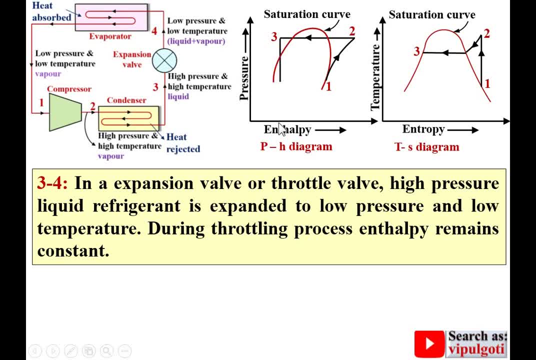 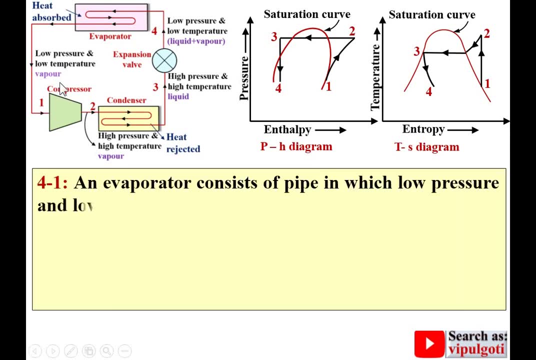 then it will be like that enthalpy remains constant. so here it is 3: 4. on the TS diagram it is the curve, and then it will enter into the evaporator. so the next process is 4: 1. so an evaporator consists of pipes. you can 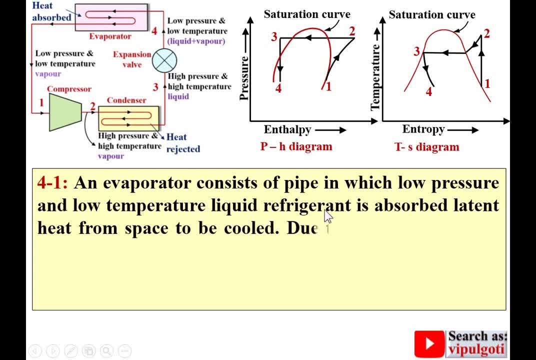 see over here in which low pressure and low temperature liquid refrigerant is absorbed- latent heat. here you can see from the space to be cooled and that is the deep freezer actually in the domestic refrigerator. due to the absorption of heat, liquid refrigerant is converted into the saturated 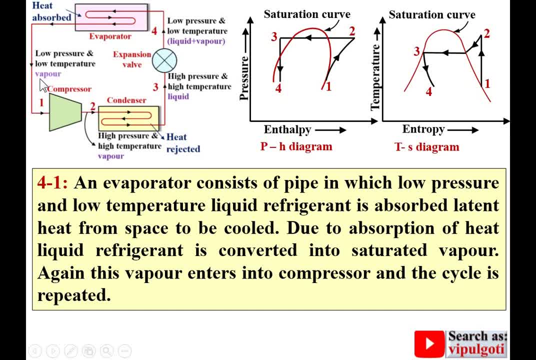 vapor, so that this mixture is now converted into the vapor again. this vapor enters into the compressor and thus the cycle is repeated. and if I want to draw that 4: 1 process on the pressure enthalpy diagram, then it will be like that, and on TS diagram it will be like that. now, next, the advantages of VCRS. first, 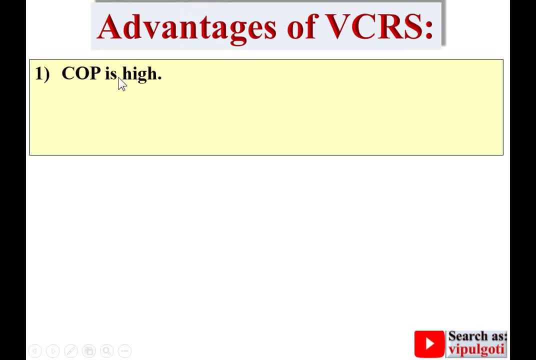 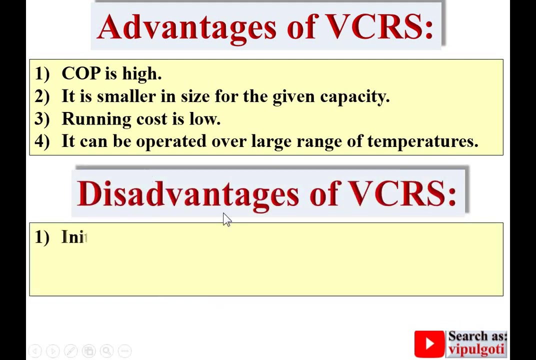 COP is high. that means coefficient of performance is high. if you compare with the other refrigeration system, it is smaller in size or the given capacity. third, running cost is low and fourth one, it can be operated over large range of temperatures. now disadvantage is of VCRS. first, initial cost is high. second, 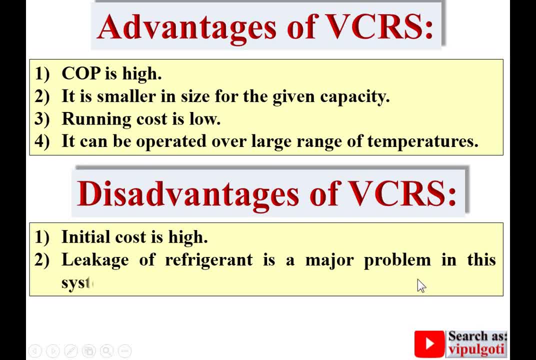 leakage of refrigerant is a must to deprive the refrigerant of temperature to the previous trabajage of VCRS. the second leakage of refrigerant is a major problem in this system because of it uses the compressor and so that the pressure is high, and thus the leakage of the refrigerant is a major problem. so 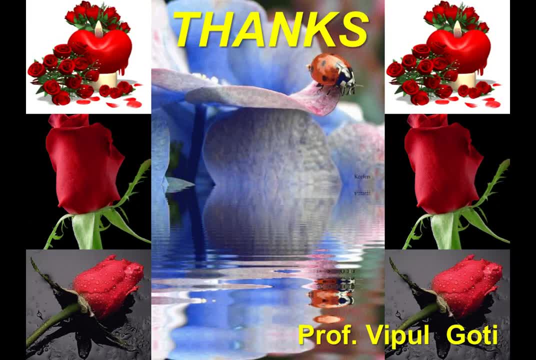 thanks, my dear friends. press the like button to appreciate this video.